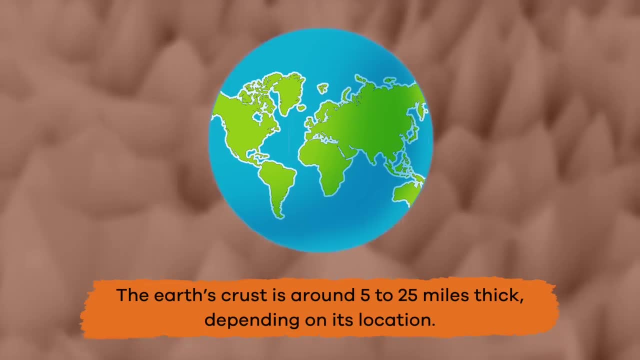 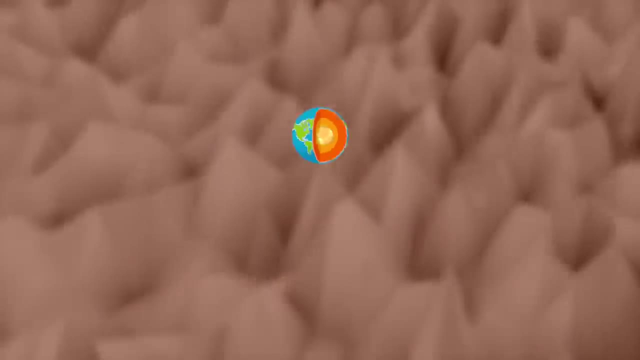 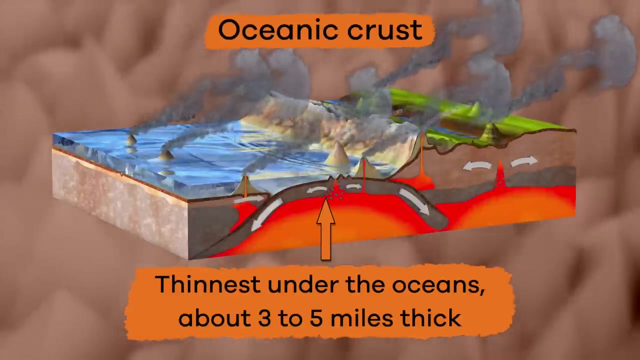 This is because you walk on it every day. The Earth's crust is around 5 to 25 miles thick, depending on its location. It is the thinnest under the oceans, about 3 to 5 miles thick, and is called oceanic crust. 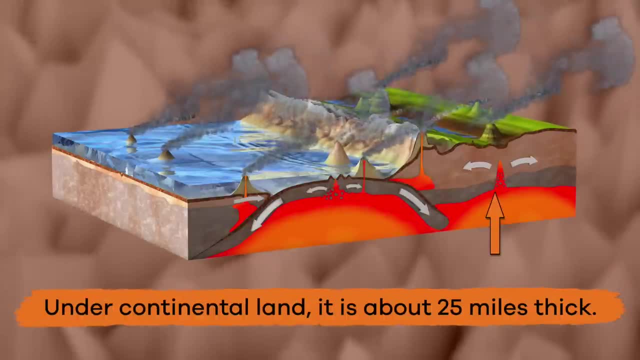 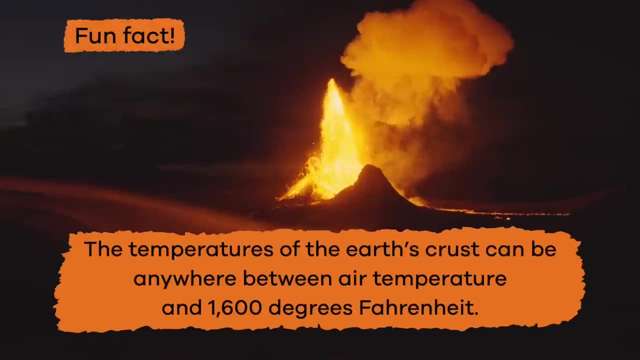 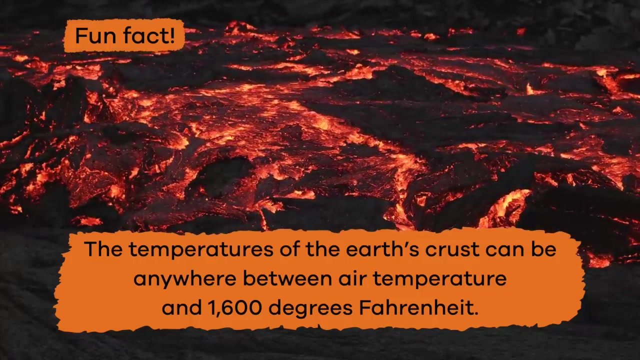 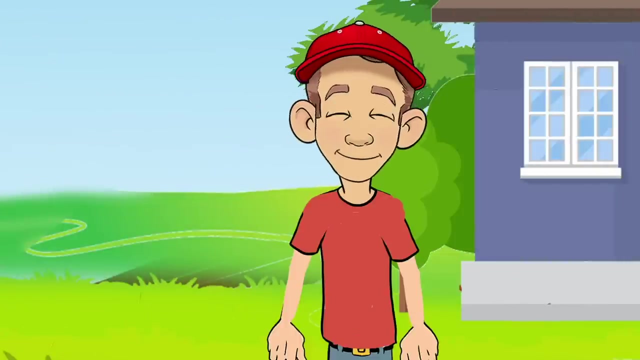 Under continental land. it is about 25 miles thick and called continental crust. Fun fact, The temperatures of the Earth's crust can be anywhere between air temperature and 1,600 degrees Fahrenheit. That is hot enough to melt rocks. The crust is also broken into pieces, called plates. 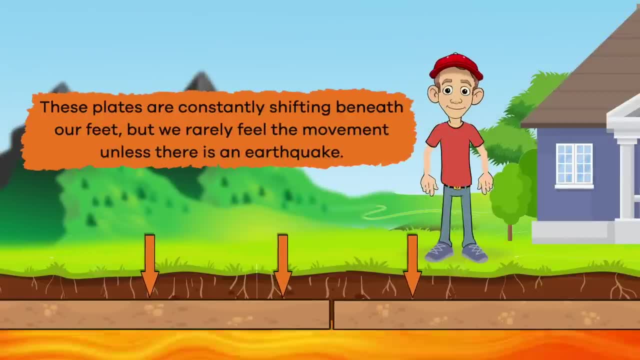 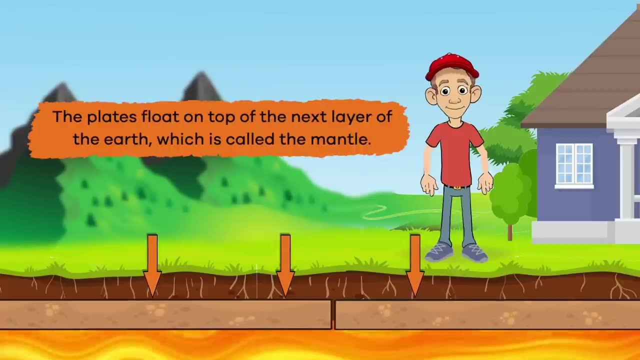 These plates are constantly shifting beneath our feet, but we rarely feel the movement, unless there is an earthquake. This is because the plates float on top of each other and the earth floats on top of the next layer of the Earth, which is called the mantle. 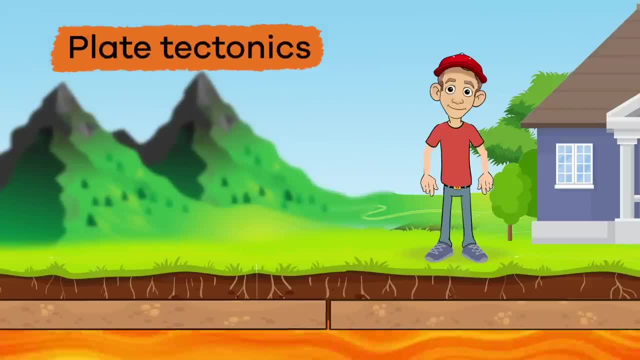 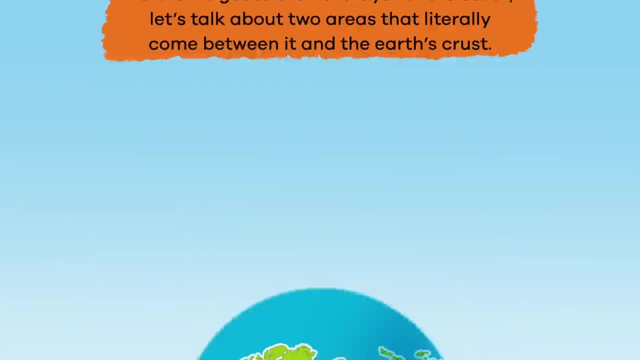 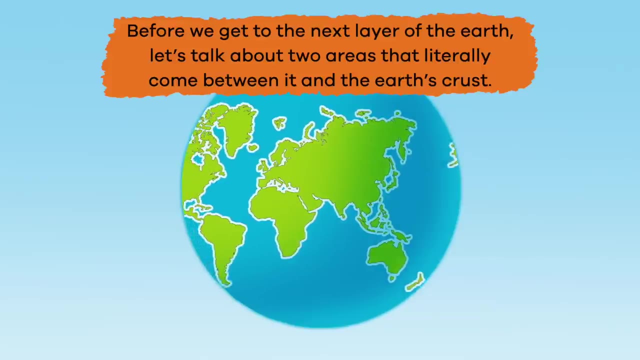 Sometimes this movement, also called plate tectonics, creates earthquakes. Whoa, Hold on to your hats. Before we get to the next layer of the Earth, let's talk about two areas that literally come between it and the Earth's crust. 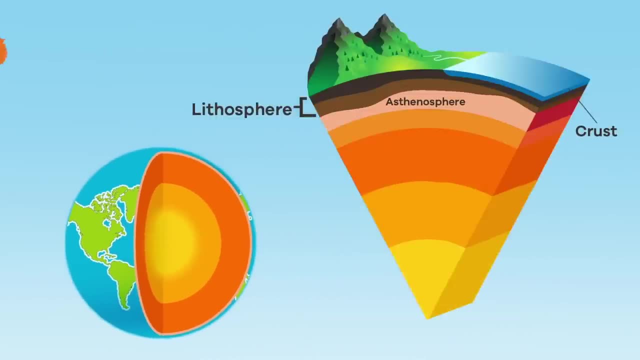 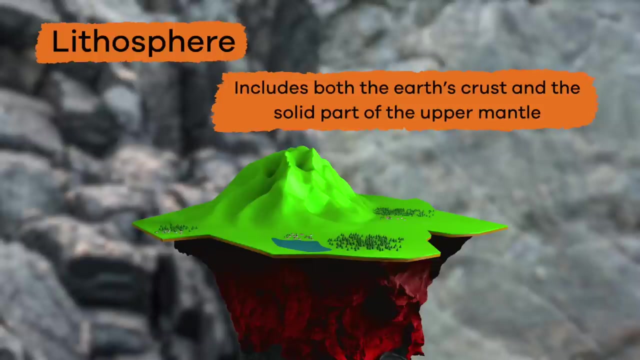 the lithosphere and the asthenosphere. Both are made up of mostly granite and basalt, but both have different roles or purposes. The lithosphere is made up of solid and rigid rocks and includes both the Earth's crust and the solid part of the upper mantle. 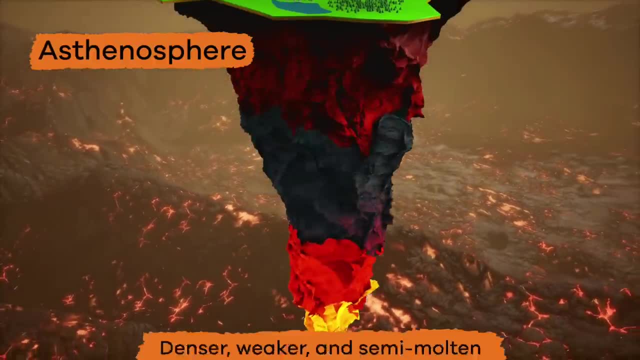 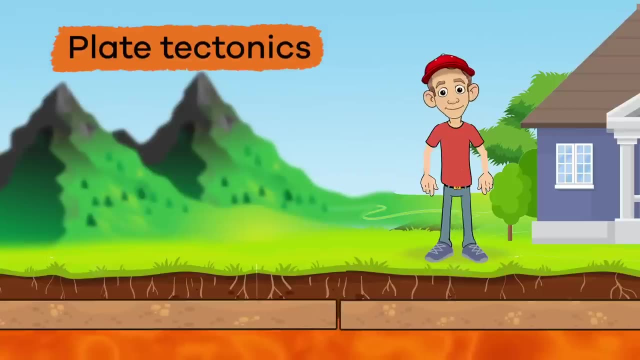 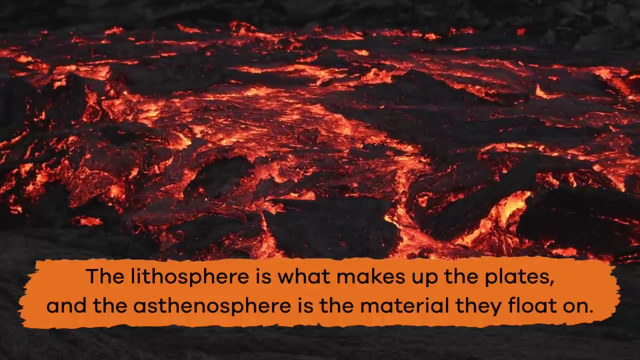 Beneath this area is the asthenosphere, which is the denser, weaker and semi-molten part of the upper mantle. Remember how we talked about plate tectonics? The lithosphere is what makes up the plates and the asthenosphere is the material they float on. 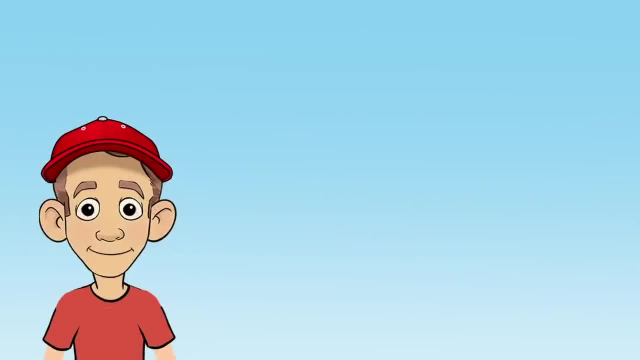 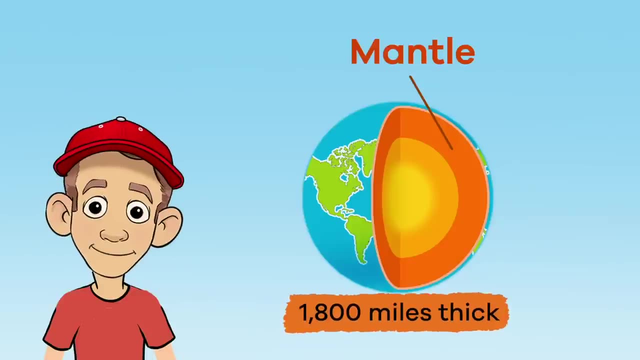 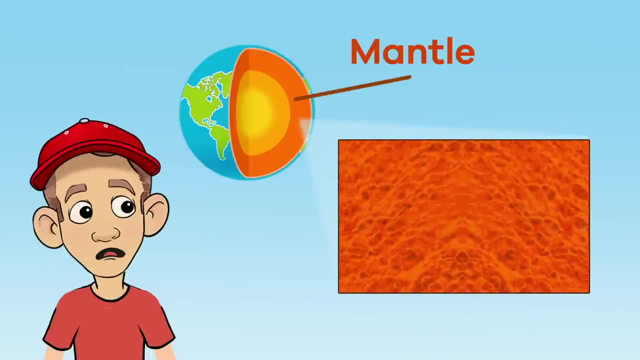 Pretty cool, right. The second layer of the Earth is called the mantle. The mantle is the planet's largest layer and is about 1,800 miles thick. It is made up of extremely hot, dense rock called magma, which flows like asphalt. 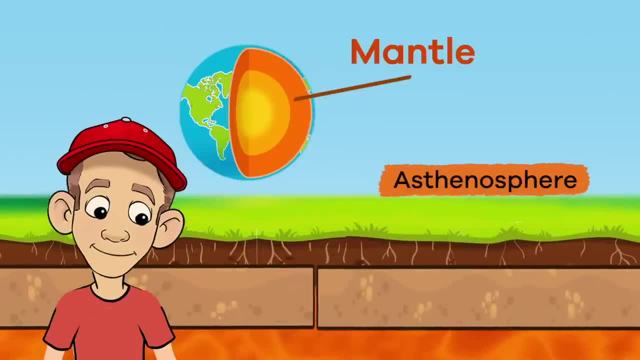 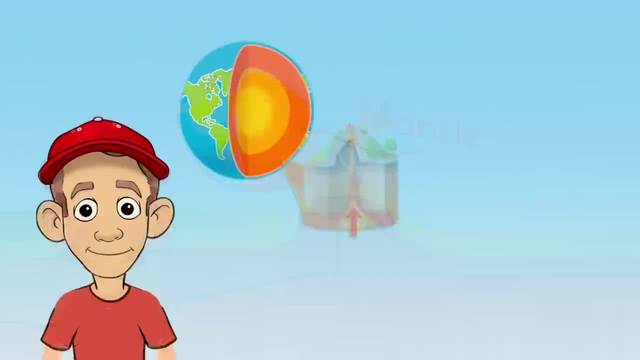 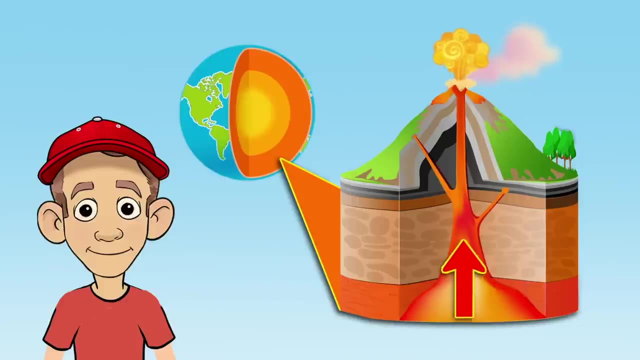 This magma is part of the asthenosphere, which is the surface that the plates of the Earth's crust float on that we mentioned before. The melted rock that escapes to the Earth's surface is what creates volcanic activity on the Earth's surface. 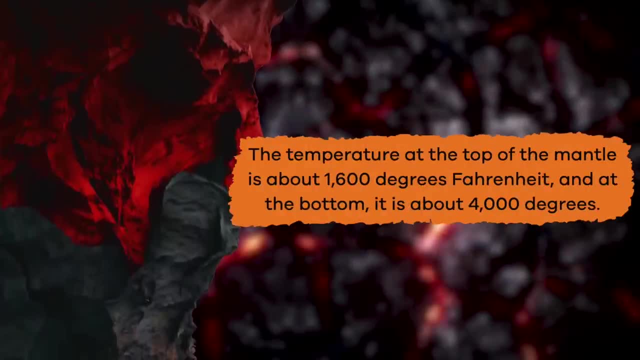 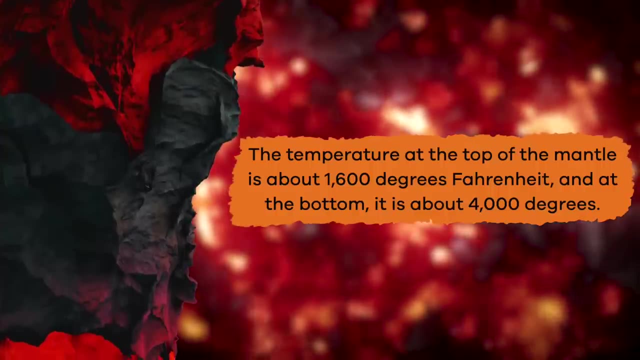 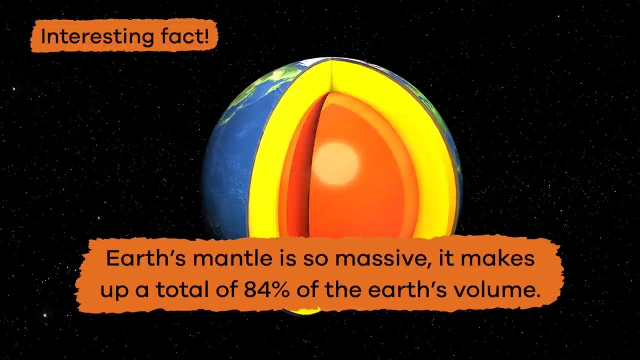 The temperature at the top of the mantle is about 1,600 degrees Fahrenheit and at the bottom it is about 4,000 degrees. Here is an interesting fact about the Earth's mantle: It is so massive. it makes up a total of 84% of the Earth's volume. 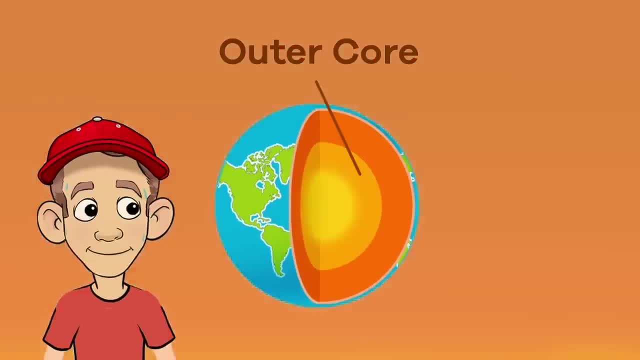 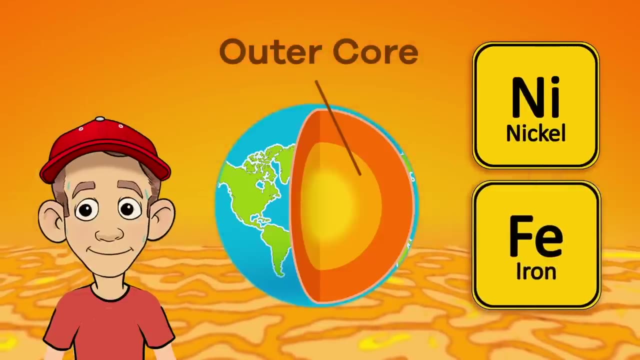 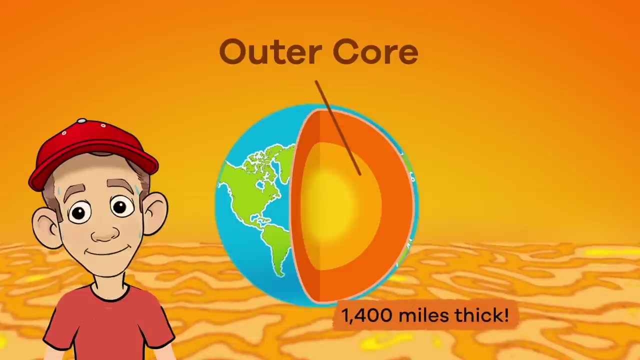 Next up is the outer core, which is basically made up of two melted metals, nickel and iron, that move together as a liquid. The outer core is located about 1,800 miles below the Earth's surface and is about 1,400 miles thick. It has temperatures between 4,000 and 9,000 degrees. Last up is the inner core, which is just as hot as the hottest parts of the outer core, but with a lot more pressure. Here is an interesting fact: This pressure comes from the other layers of the Earth. 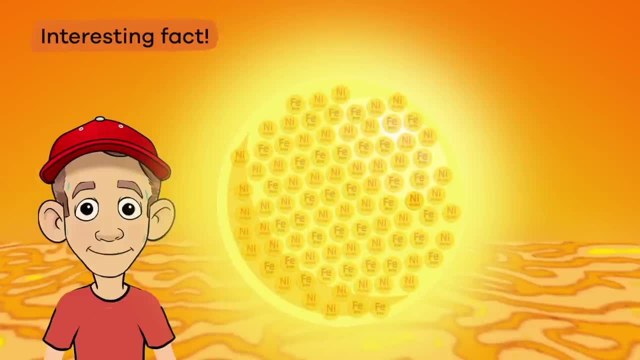 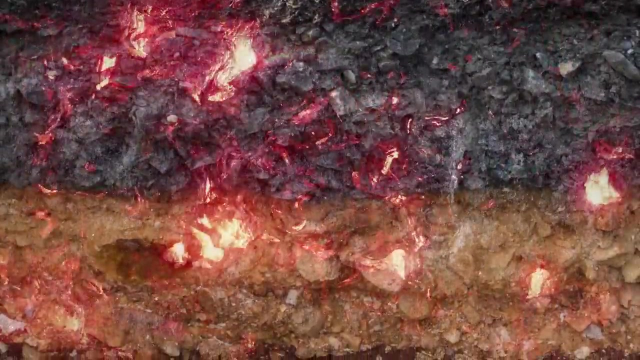 pressing down onto the inner core, Which causes molten iron and nickel to be so tightly forced together that they are forced to vibrate as solids. Who knew that was even possible? Now that we have dug deep into the Earth's layers, let's see what you can remember. 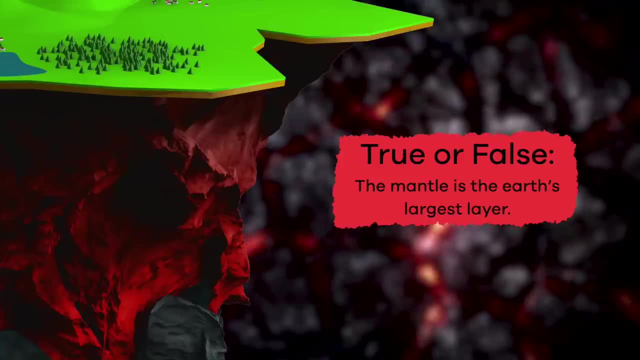 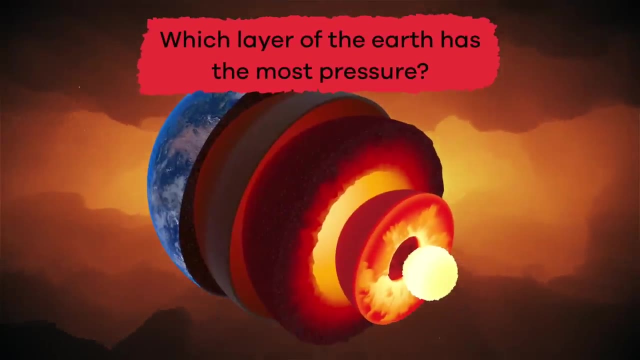 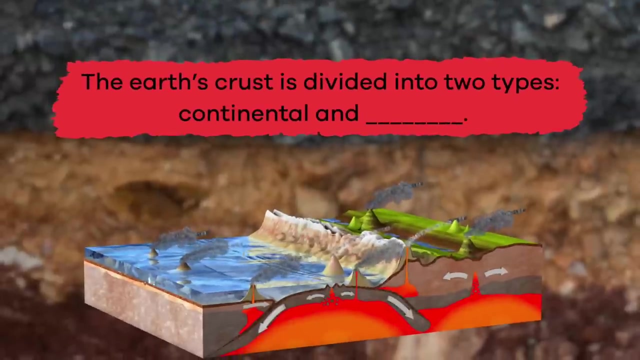 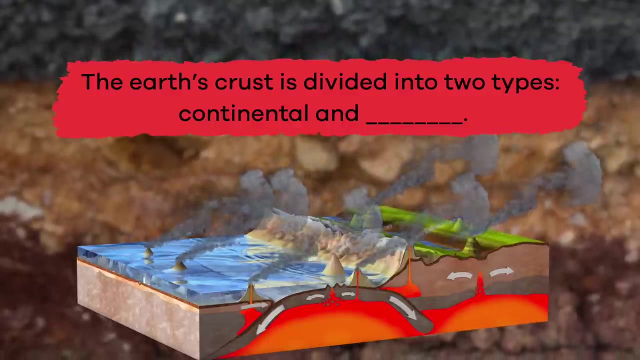 True or false, The mantle is the Earth's largest layer. True, Which layer of the Earth has the most pressure? The inner core? Fill in the blank. The Earth's crust is divided into two types: continental and blank Oceanic. 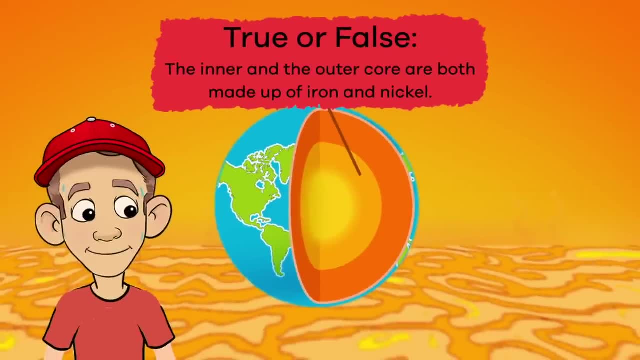 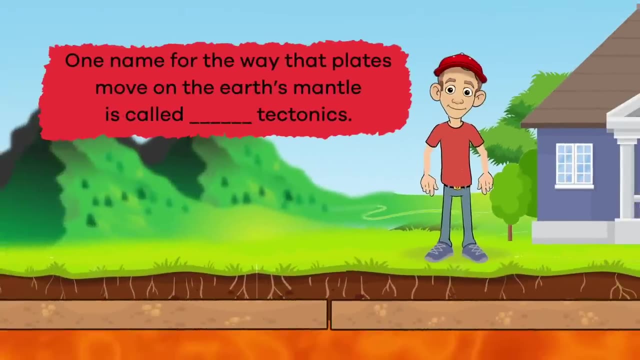 True or false, The inner and the outer core are both made up of iron and nickel. True Fill in the blank. One name for the way that plates move on the Earth's mantle is called blank tectonics Plate. Great job, friends. 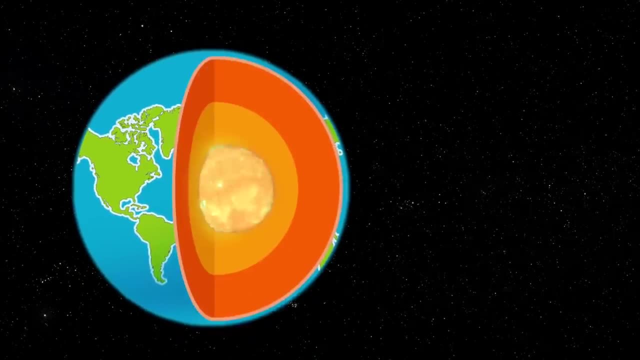 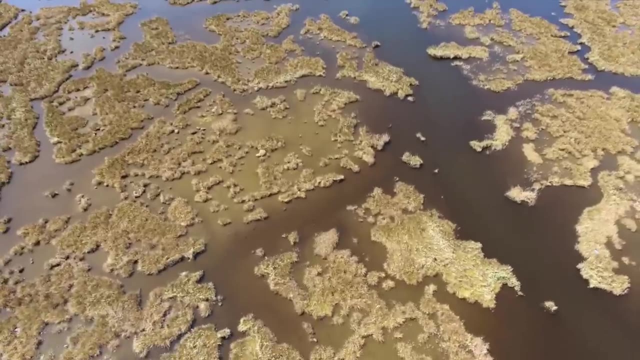 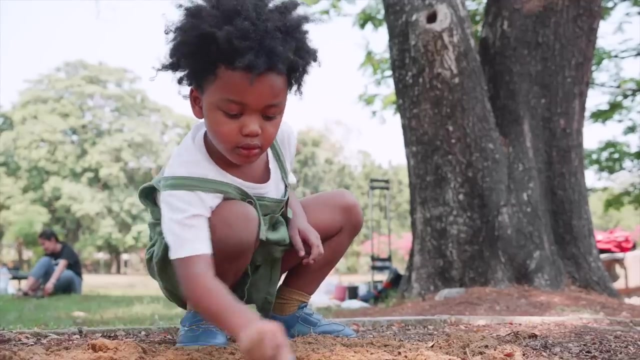 The Earth is a massive planet with four main layers: the crust mantle, inner core and outer core. The next time you are outside, take a minute to examine the ground you are walking on, and maybe even take a minute to dig a hole in the ground.